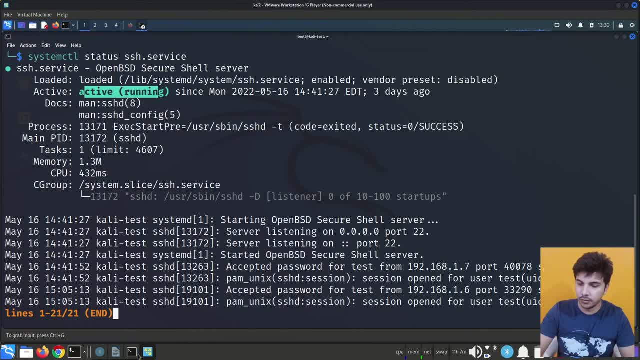 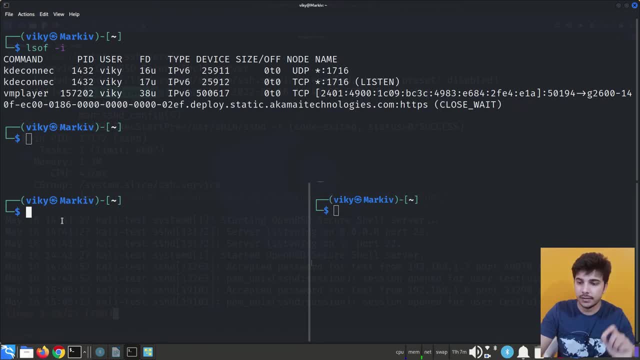 this service is running at this moment. so what i am going to do, from my host system i am going to make a connection, that is ssh connection, to this particular system. so i will write here ssh, then test at the rate 192.168.1.6. 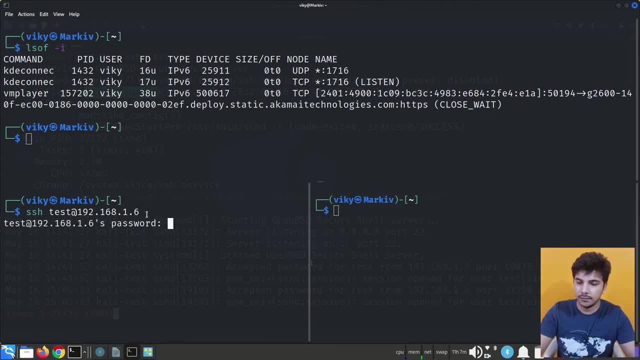 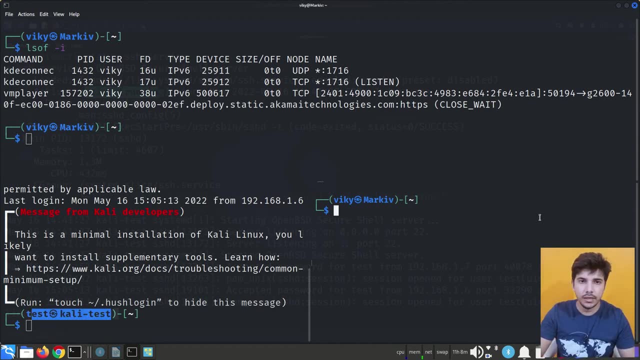 let's press enter and it will ask me for the password. so let's give the password and the connection has been established. now i will also make a connection to one of the open ftp servers. so in the google you can type out that list of open ftp servers and from there you can select any server and connect to it. 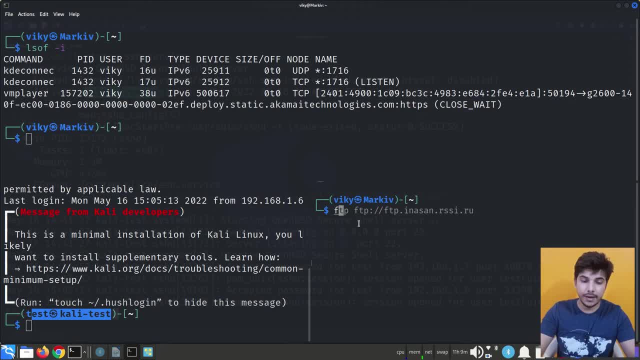 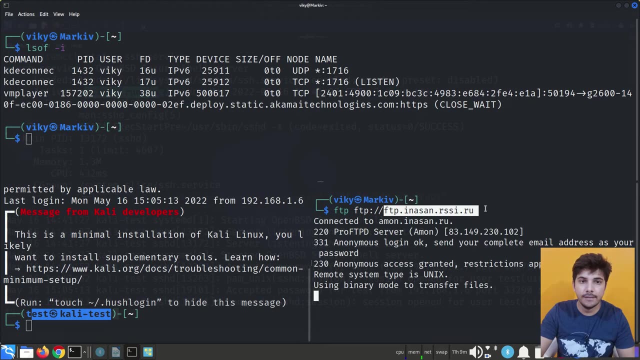 without any password. so i am going to give here ftp and will provide the server url with the ftp protocol, and it is going to connect me with this particular ftp server without any password, just like this url. there are lot of urls that are openly available, right? so this connection has 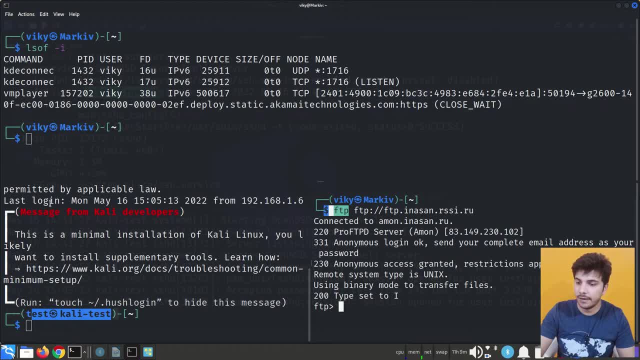 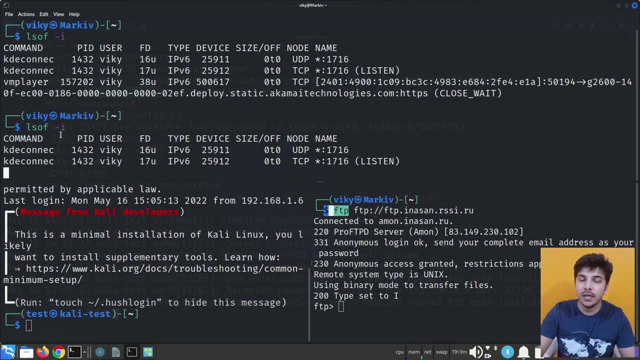 been established. so we have one ftp connection and we have the one ftp connection and we have one ssh connection. and if we run the same command here- lsof, and then the dash i, you will see that in the connection list these connections will be shown along with their 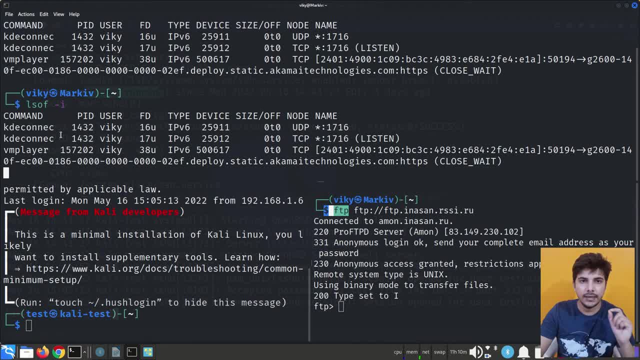 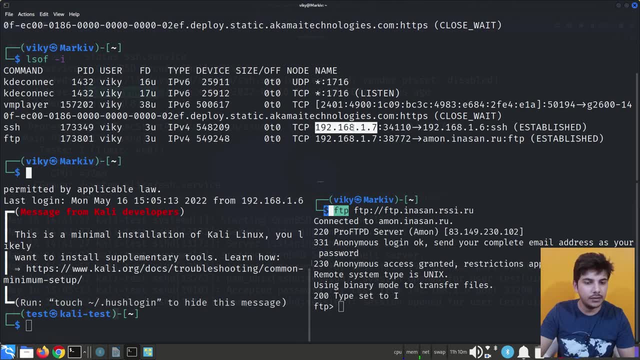 source ip and source port and destination and destination port. so if we view the output then we will notice that from our source ip, that is 192.168.1.7, and from the source port, 34110, we have established a connection to the 1.6, that is a local system in our private network and the protocol is ssh. similarly, we had 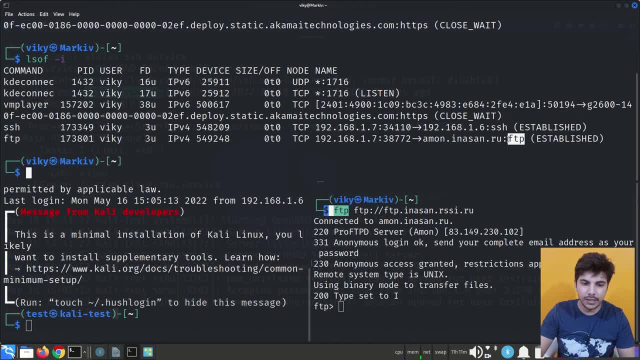 made another connection with the protocol as ftp right. in both of the cases we are able to see the source port and also the destination protocol. now, by default, it is giving us the domain name and also the protocol names, but let's say we don't want to show them rather than giving it. 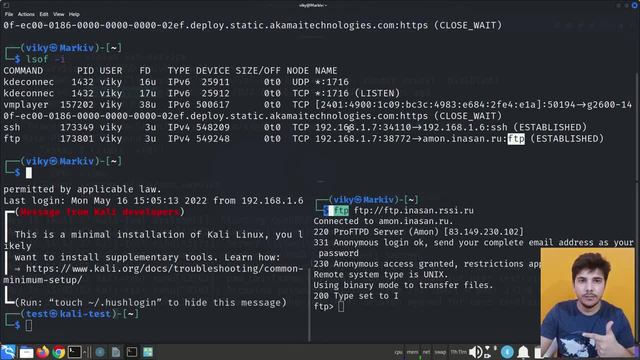 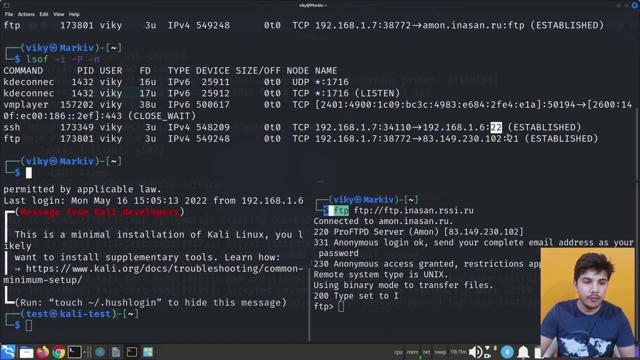 we want to have the proper ip address and instead of protocol we need to define the port number. so for that we can give the option here as dash capital p and also the dash n. so in this case you will see, the port number for the ssh is 22, while for the ftp connection it is the 21, and we will notice that url is also in the ip. 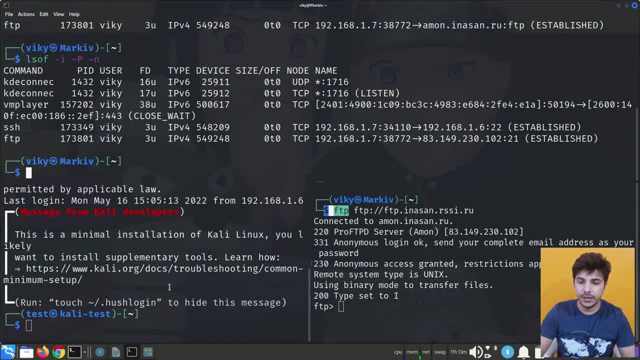 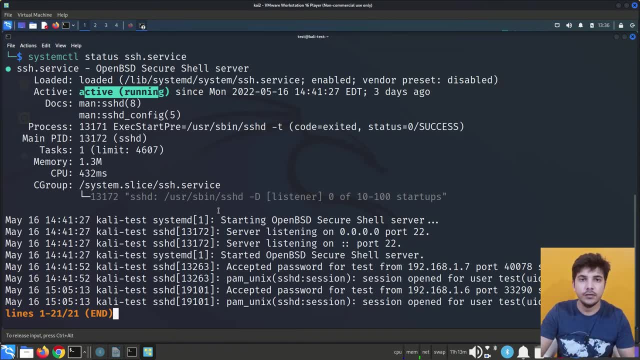 form. right now let's see the second section of the video, in which we are going to make a connection to the local system and we are going to make a connection to the port number and we are going to make a connection to the local system present in our private network, and we will notice that the 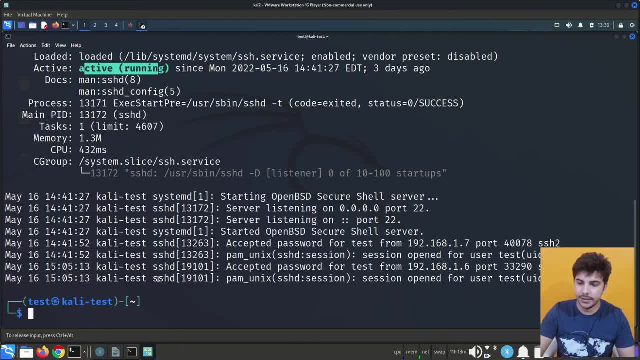 source address and the source ports are not getting translated. for that we have hosted a website into this dot 6 server and the website will tell us what is the source ip address and what is the source port number. so if we view the content of the files that are hosted into this, 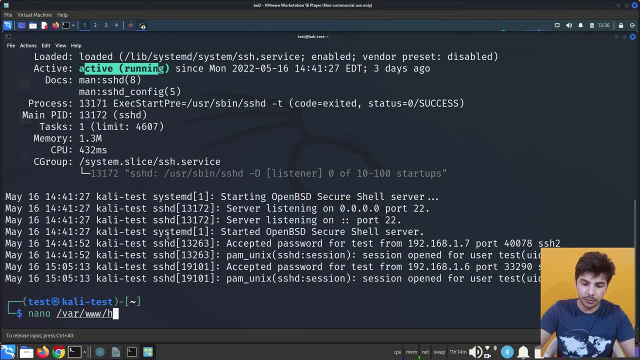 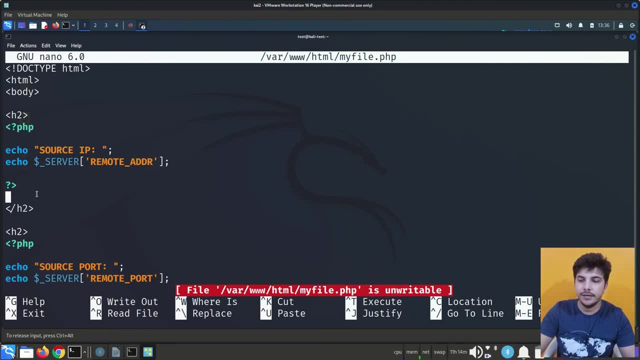 web server. so let me go to the where www html and also the my file dot php. so into this file we will notice that we had written a very basic php script that will give me output as source ip and it is going to print me the remote address. remote address means that it. 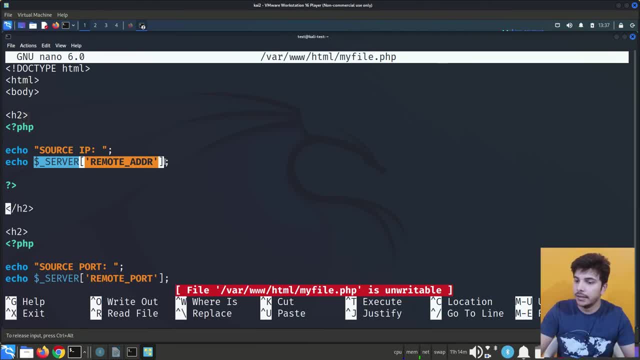 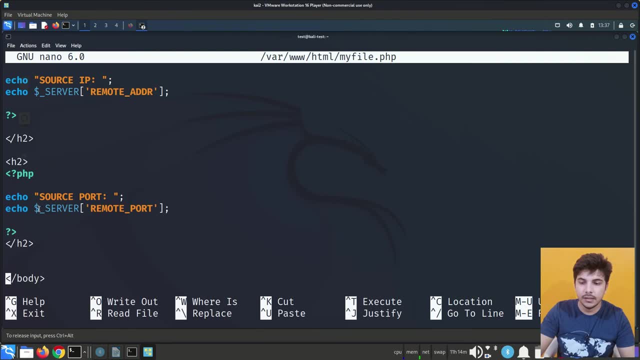 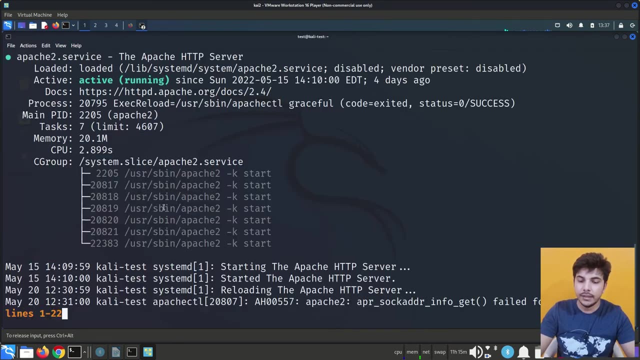 will give the ip that is making the connection now. beneath that, we will see that again, we had written a very short php script that will tell us the remote port right and at this moment, if we view that the apache is running, so our web server is also running. now, if we open up the chrome browser, 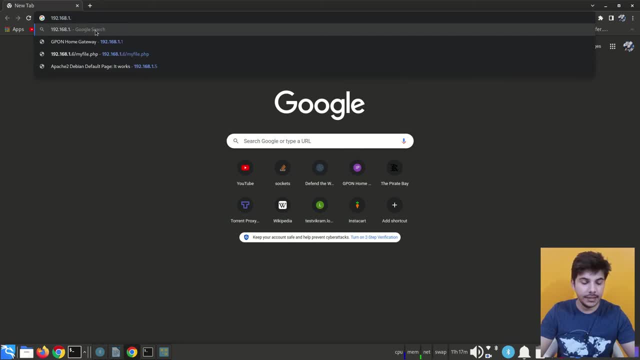 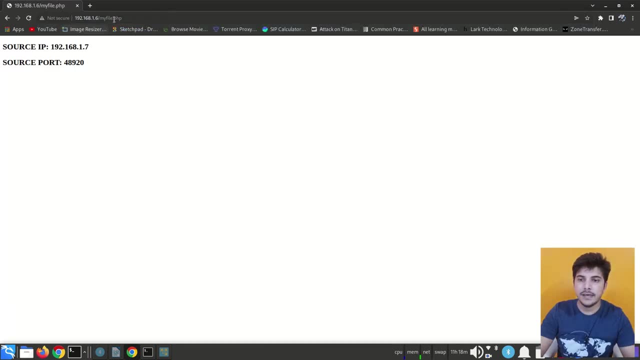 and let's make a connection to that system that has the ip address as 192, 168, 1.6, on which our web server is running, and the file name is my file, dot php. so it will give me the source ip address that is making the connection. so in this case it is dot 7 and the source port number right. and if 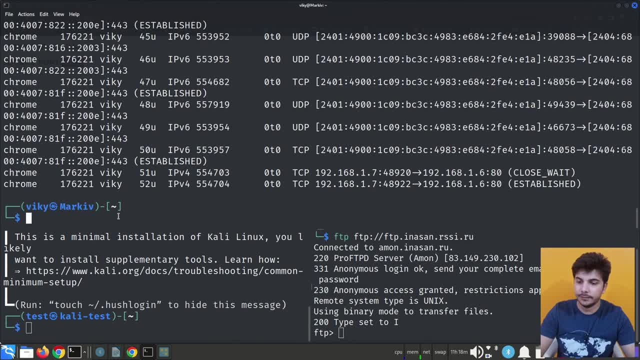 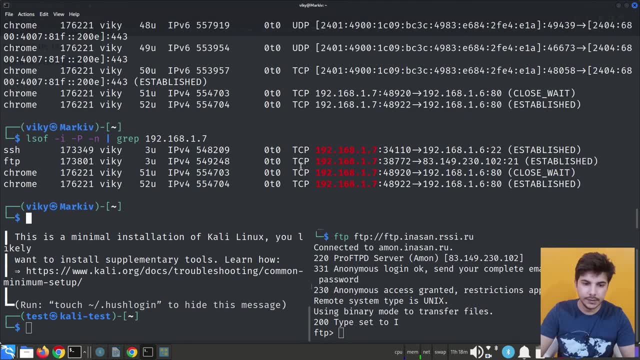 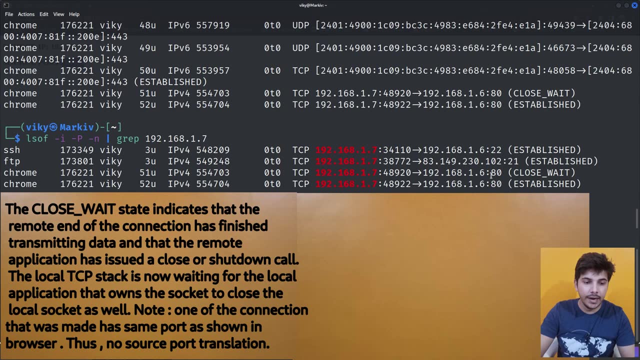 we go to our terminal and give the same command right and let me grab here 192 dot 168, dot 1.7, right. so in this particular case you will notice that various connection is being made from our system and one of the connection was from dot 7 to dot 6 on port number 80. so basically, whatever the connection we are, 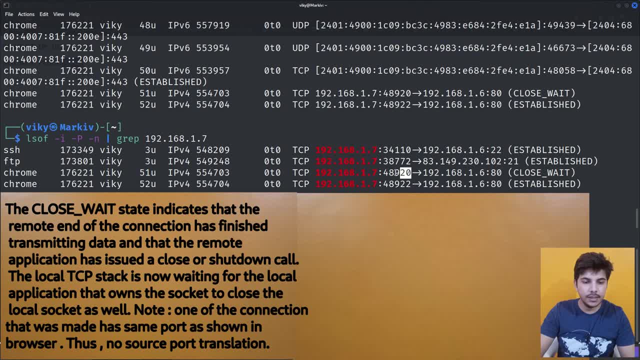 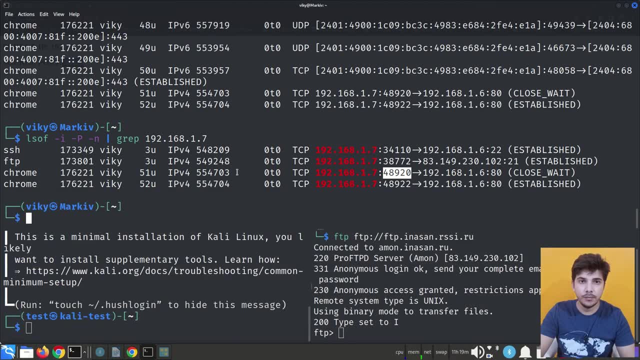 making to our web server. so in this particular case, the port number 48920 has been used. now let's see the third section of the video, in which we are going to make the connection to outside of the private network, and we will notice that our source ip and source port will. 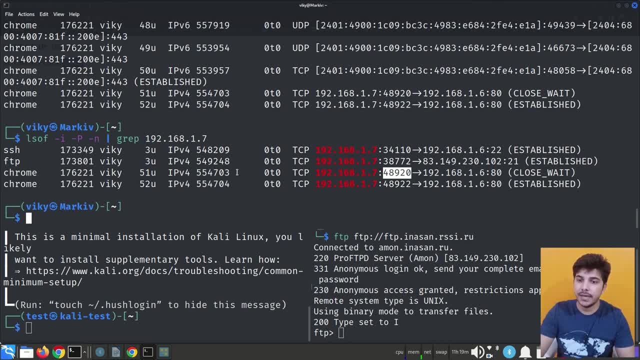 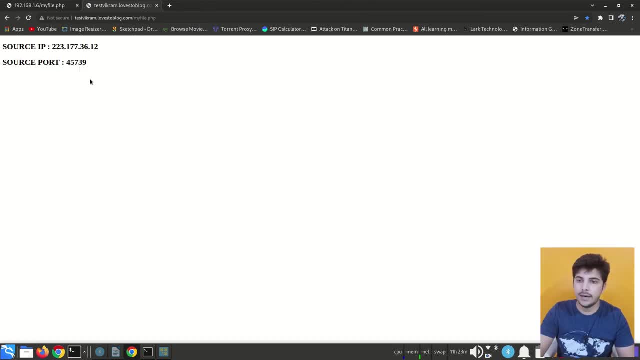 get translated. so i have hosted the same website into a public domain right, which will also give me the same output that what is the source ip address and what is the private ip address. so currently my source ip address, if you will see it, is showing 223 178 and i have hosted the same 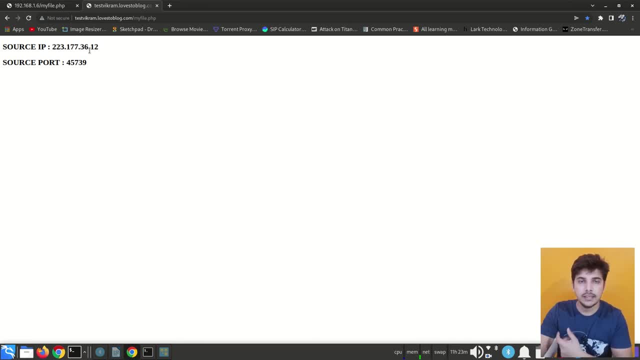 website into a public domain right, so i have hosted the same website into a public domain right. so any connection that i am making outside of the internet between them, our router is changing the private source ip with the public ip address. similarly, my source port is also getting. 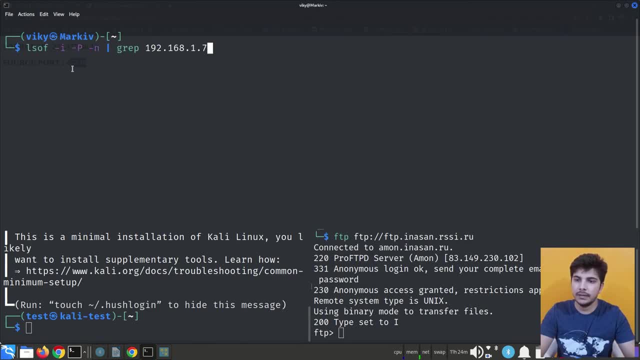 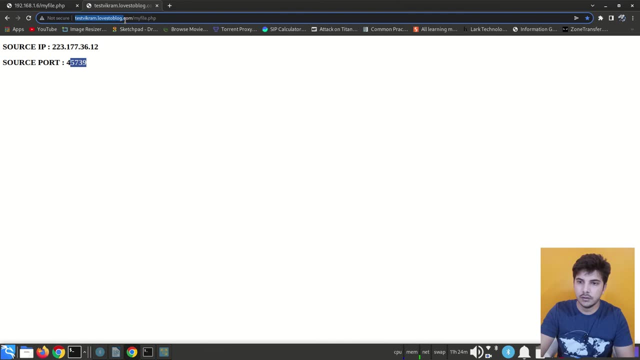 translated for that we will run the same command, that is, lsofi dash i capital p? n. so what i am going to do, let's resolve this particular host name to find its equivalent ip. so i am going to write here host name and i am going to write here host name and i am going to write here host name. 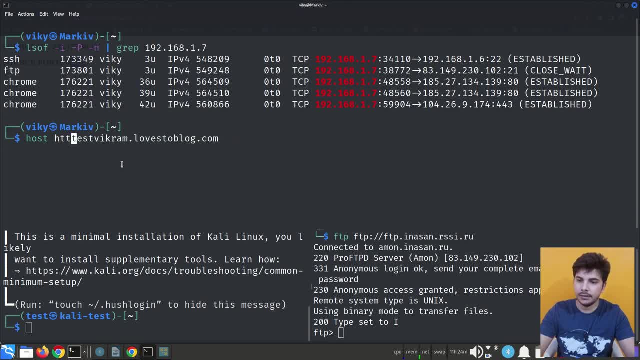 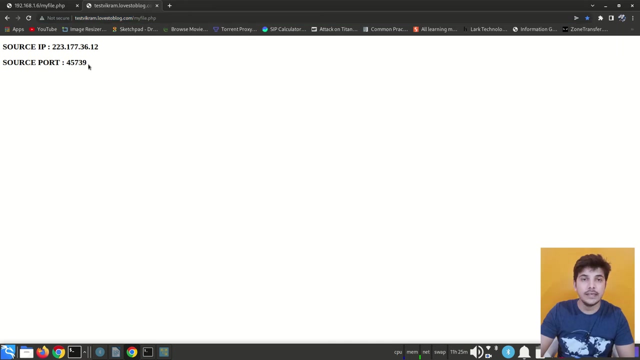 and then the domain name right. so the ip address of our server is 185.27.134.139. and here we are making some connection right. at one time we are using the source port as 48558 and in the another time we are using the 60, but no such port has been shown here. why it is happening? because the router in between. while doing the path that is port address translating, is changing my source ip address and also changing my source port address. that is the reason when this particular web server that is residing into the public network gets this connection. it is having the source port different to the source port defined by my system right now. 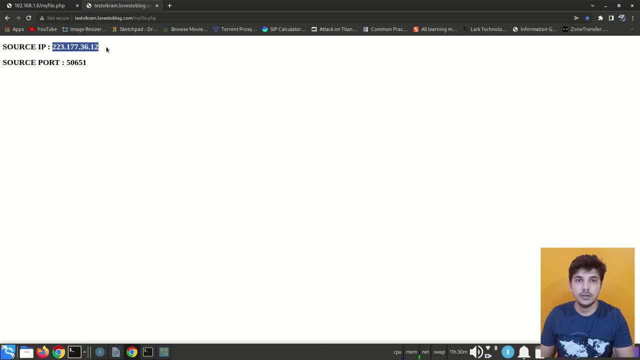 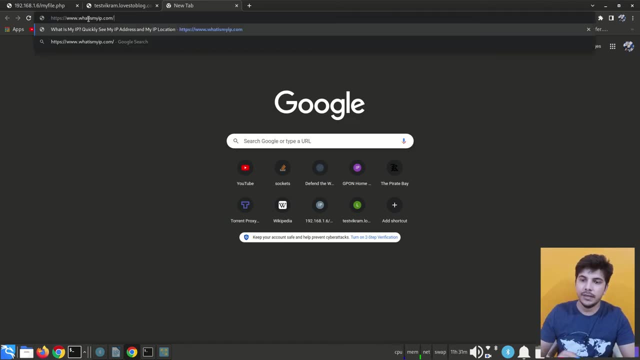 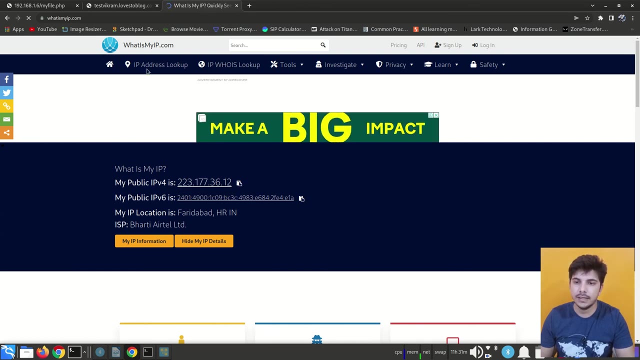 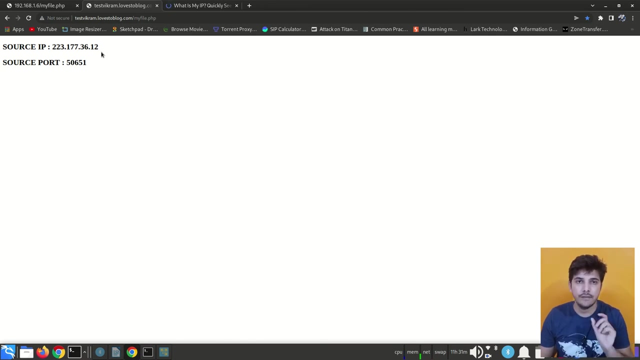 here. the ip address is 223.177.36.12, because this is my public ip address, i give here. what is my ip address then it is going to give me the same public ip address, that is, 223.177.36.12, and the same has been provided by the web server, right. so with that we can conclude that whenever 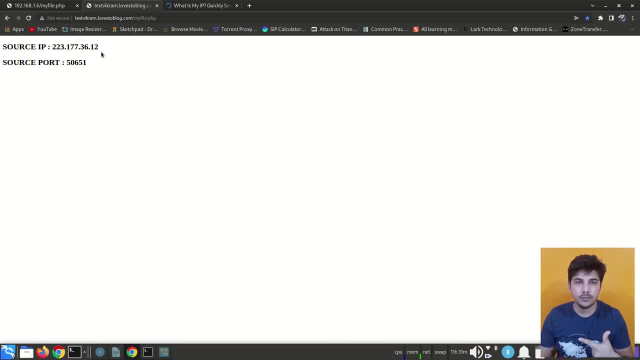 the pat is happening, then our source ip and the source port is getting translated, and whenever the connection is happening within our local network, then no source address or no source port is getting translated. so that's all for today, guys. i hope you have enjoyed this video and i will see you in the next one. bye, bye, bye. 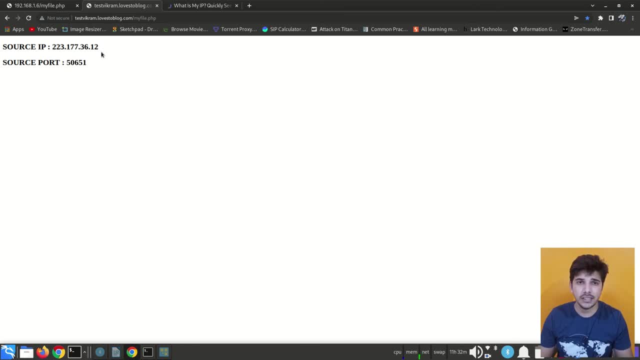 hope you like the video. if you have any doubt, please comment it down. thanks for watching and i hope to see in the next video.